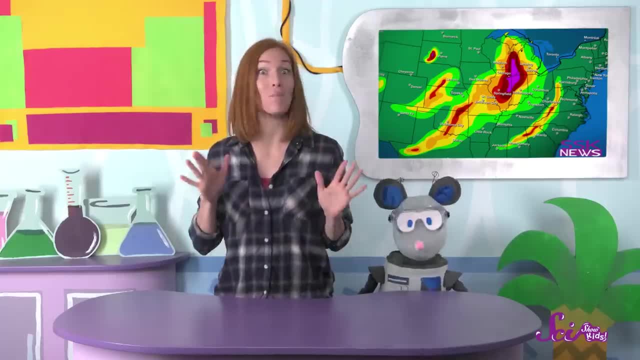 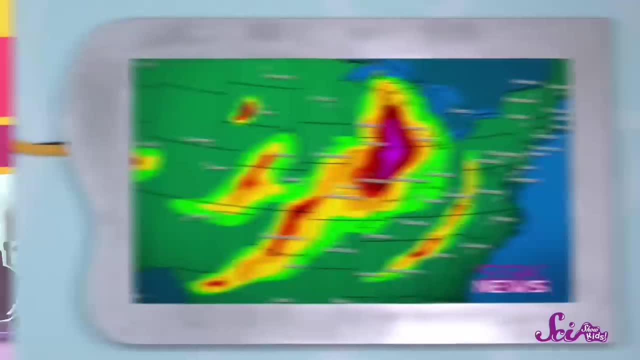 But meteorologists can look at the picture and tell lots of things about the weather. For example, the different colors on a radar picture show where it's raining and how hard it's raining: Green means a little bit of rain, yellow means a medium amount and red means it's raining. 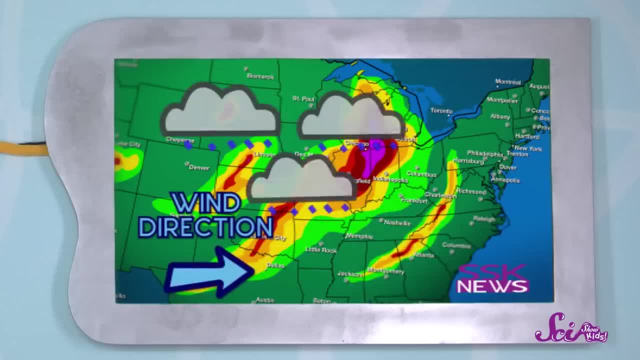 a lot. Radar also shows which way the wind is blowing and which way the rain is coming from. The radar also shows which way the wind is blowing and which way the rain is coming from. It also shows which way the rain clouds are moving. 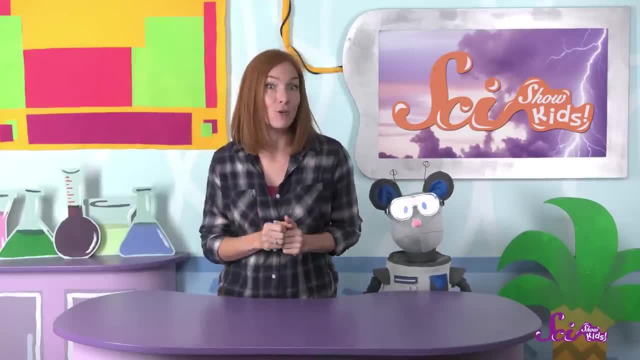 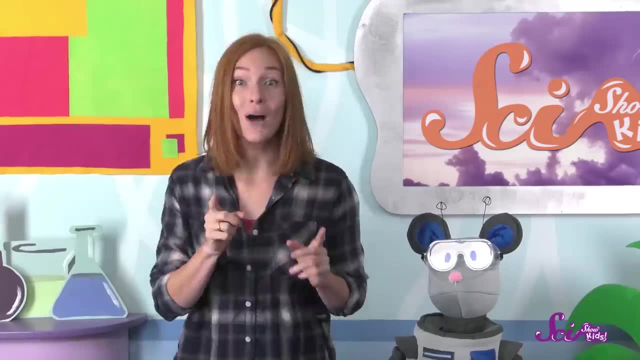 So even if there are no clouds in the sky right now, if radar shows that some rain is moving toward where you live, there's a good chance you're going to get rain pretty soon. That's one clue meteorologists can use to predict the weather. 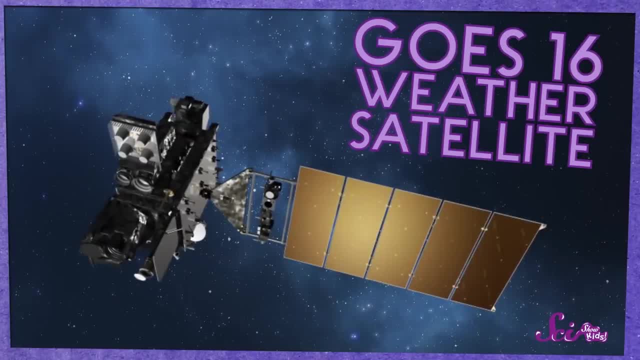 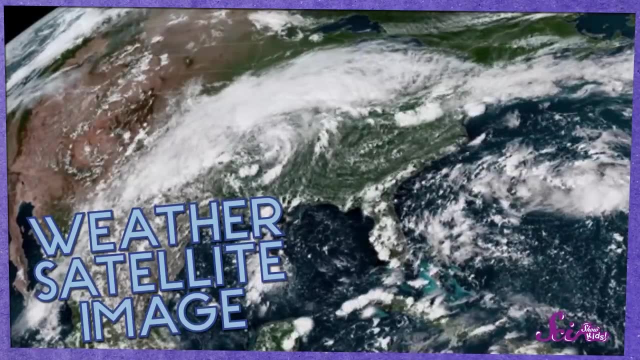 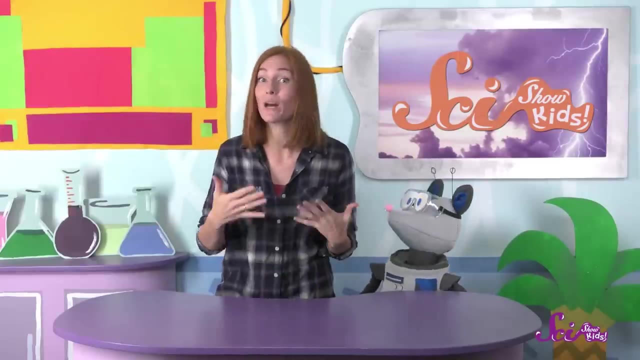 They can also use satellites- computers we send into space that can take pictures of the Earth. When meteorologists look at the pictures from satellites, they can see the clouds from above, including which way they're moving and how fast. That helps them see when storms are forming and predict where the storms will go. 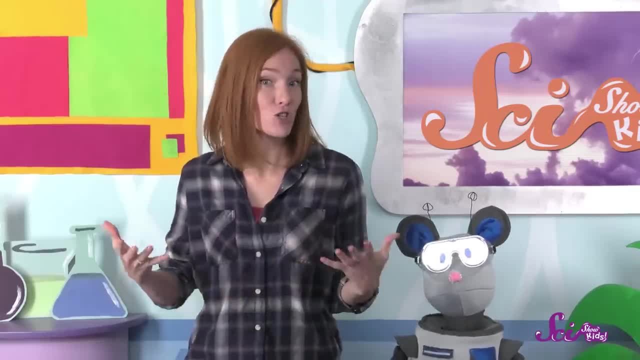 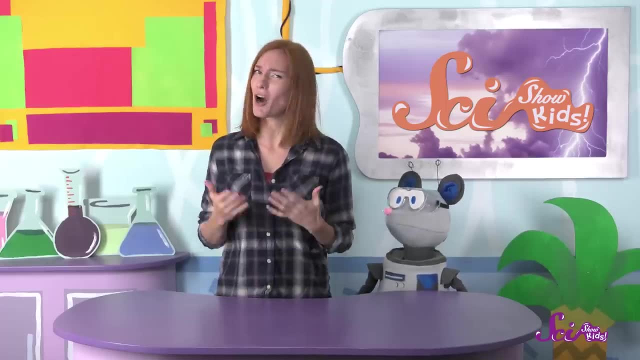 So that's another clue. If a satellite picture shows a storm is heading your way, a meteorologist can tell you that it might rain in a few days. Now, satellites and radar are pretty amazing tools, but they only provide some of the clues. 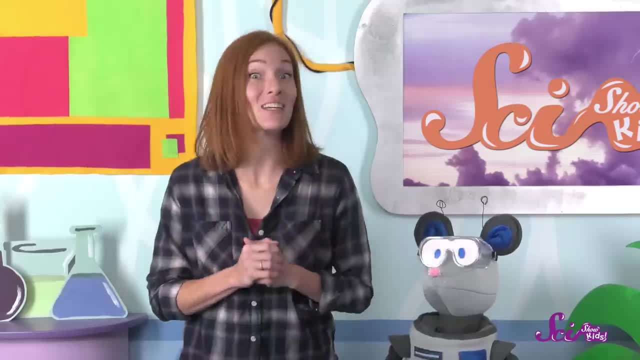 that meteorologists need to predict the weather. Meteorologists can also sometimes tell if there will be a storm before there are any clouds. Meteorologists can also tell if there will be a storm before there are any clouds. Meteorologists can also sometimes tell if there will be a storm before there are any clouds. 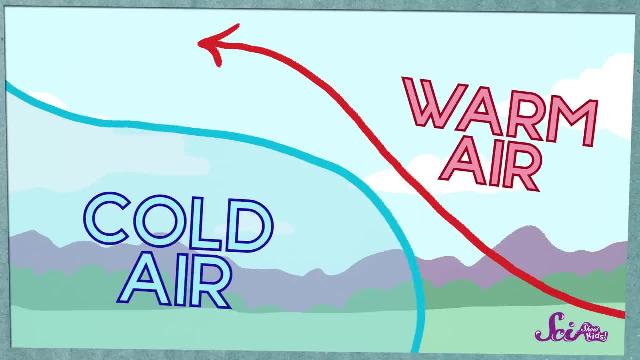 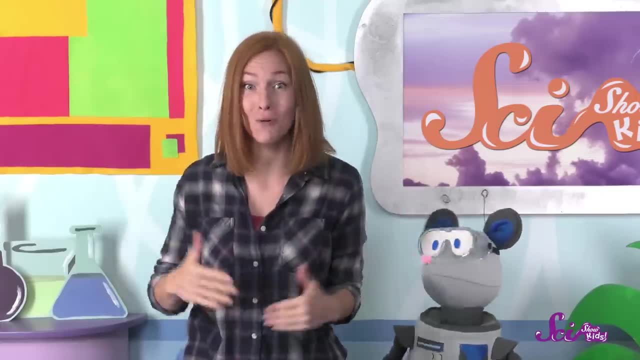 warm air meets a bunch of cold air, they usually create some clouds and rain when they mix together. So if a meteorologist sees that there's some warm air and some cold air moving toward each other, they know it will probably rain when the two types of air meet. 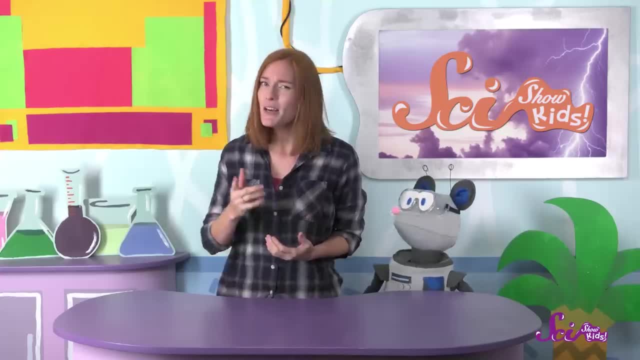 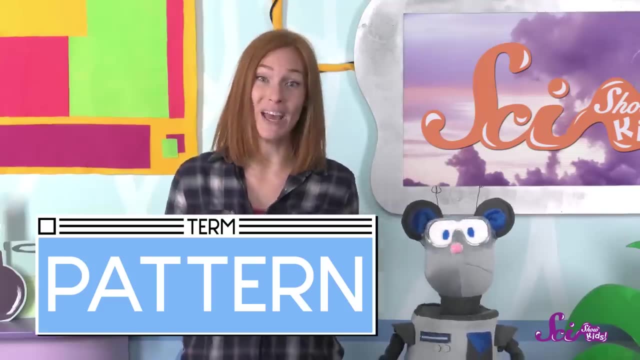 But some of the most important clues that meteorologists use come from something that you can do at home: Look for patterns. A pattern is something that happens the same way over and over again. So if you live in a place where it was hot in summer and cold in the winter last year, 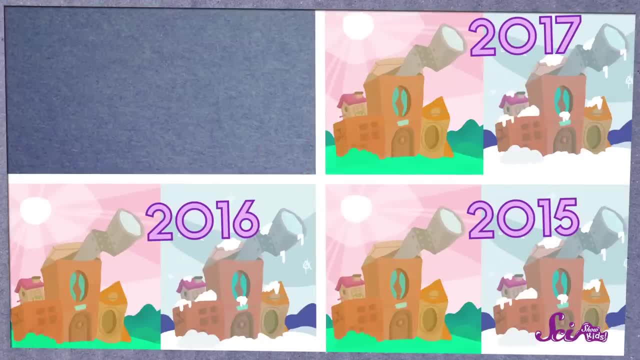 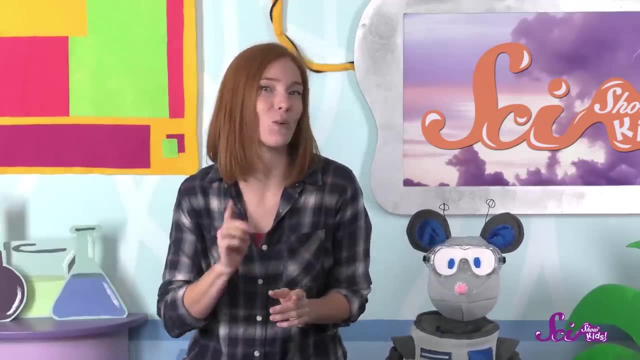 and the year before and the year before that it will probably be the same this year too. Meteorologists look at weather patterns all the time and use the patterns they find as clues when they predict the weather. Ah, you're right, Squeaks.